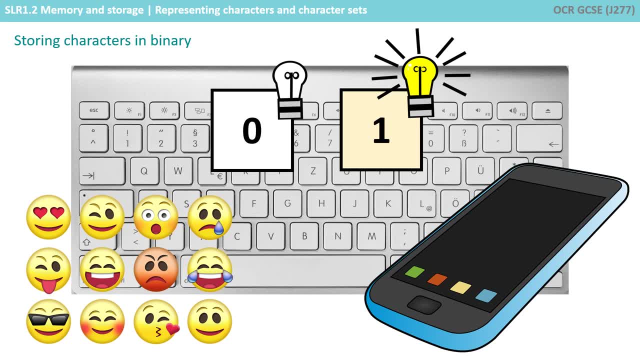 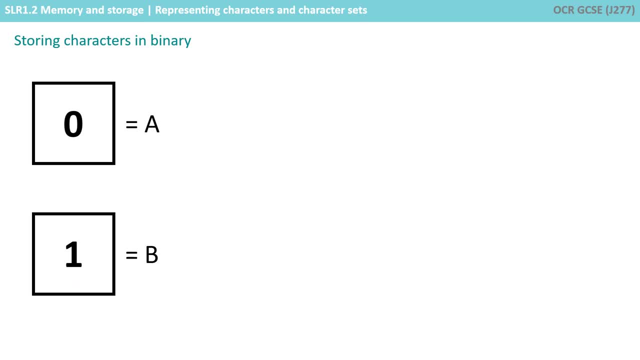 and the emojis you send in text messages must all have their own binary codes. If each character was represented by only one binary digit, then it would mean we could only store two possible characters, perhaps A and B. If we had two bits for each character, then we could store four possible characters. 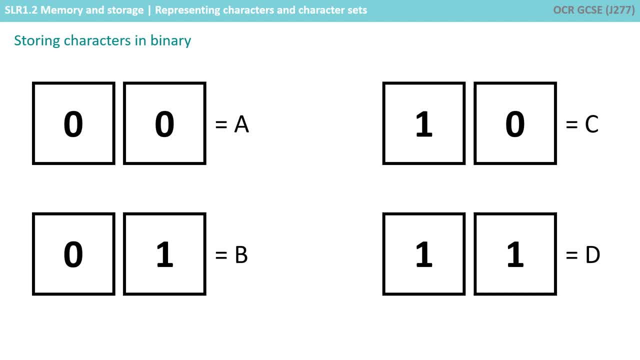 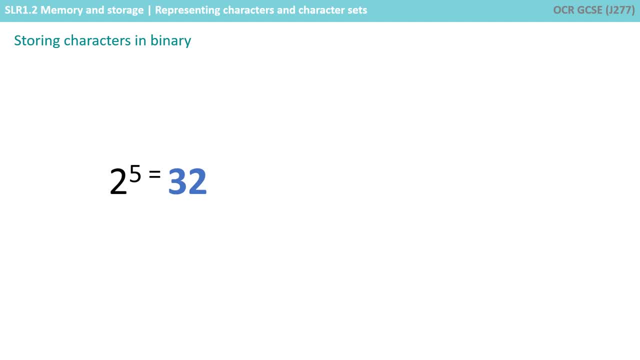 because 00 might be A, 01, B, 10B. If we had two bits for each character, then it would mean we could only store two possible characters, perhaps B, 10B, 10C and 11D. 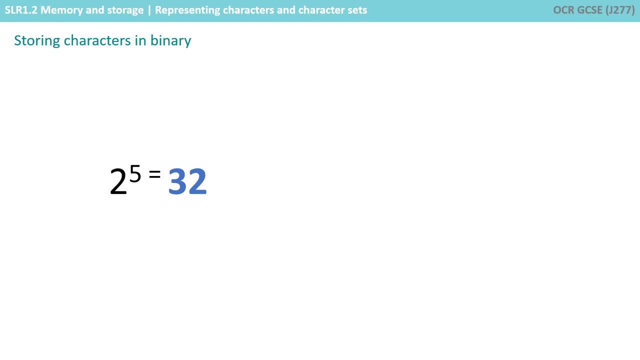 Given that there are 26 letters in our alphabet, this means that we need five bits as a minimum, which will allow us up to 32 characters. We can express the number of bits to characters mathematically. for example, 2 to the power of 5 equals 32.. 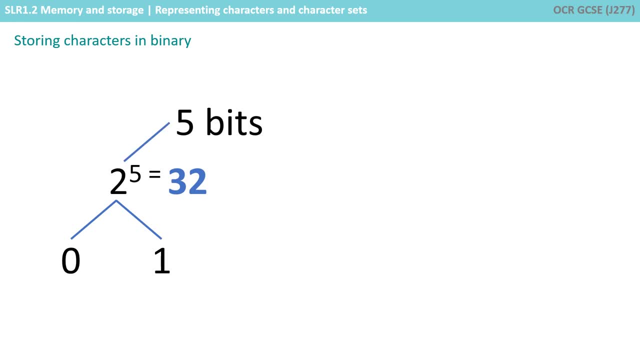 This means that the number of unique binary combinations for five bits is 32,. as each character must have its own unique code, This determines the number of bits needed to store all the characters in a set. We call this a character set, a defined list of characters. 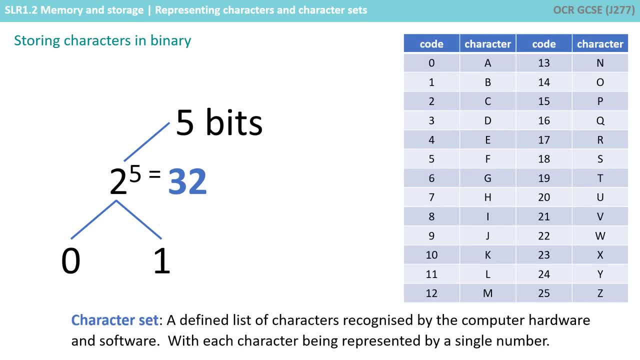 recognised by the computer hardware and software. This means that each character must have its own unique code which determines the number of bits needed to store all the characters in a set. If we had two bits for each character, we would have serviced in the software. 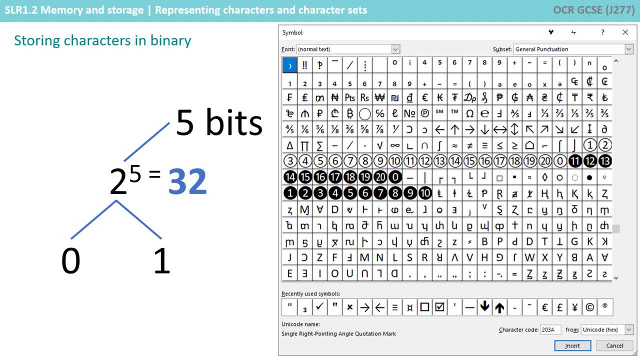 and each character represented by a number. Of course, there are more than 26 characters we want to be able to store. There are both upper and lower case letters, and that doubles the number of characters we need instantly. But there are also symbols such as pound signs, brackets and punctuations. 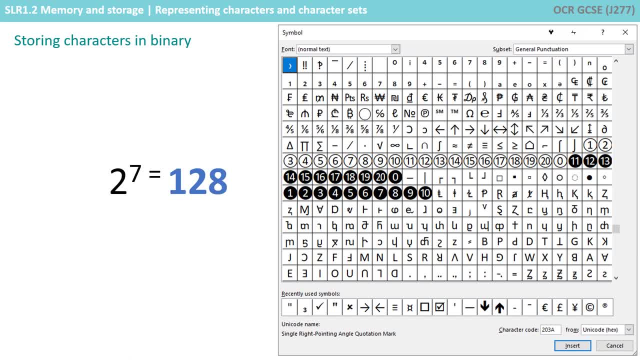 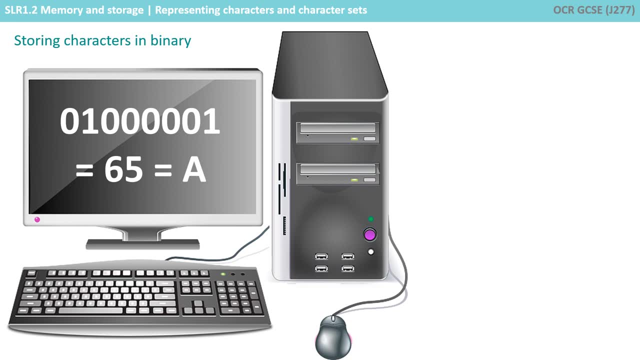 Therefore, we actually need a minimum of seven bits for each character, 128 unique binary numbers, 128 unique characters in the character set. It is important that every computer is using the same binary number to represent each character. For example, if my computer uses the code 0 1 0, 0, 0 0 0, 1 to: 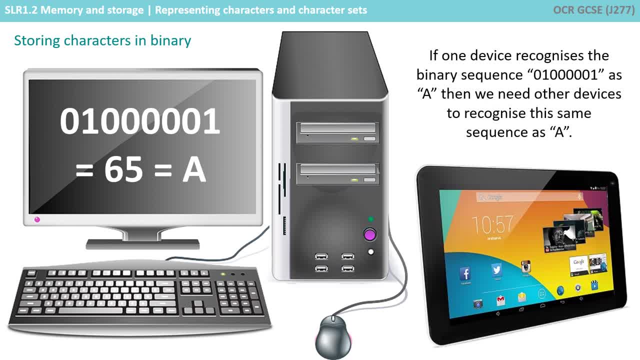 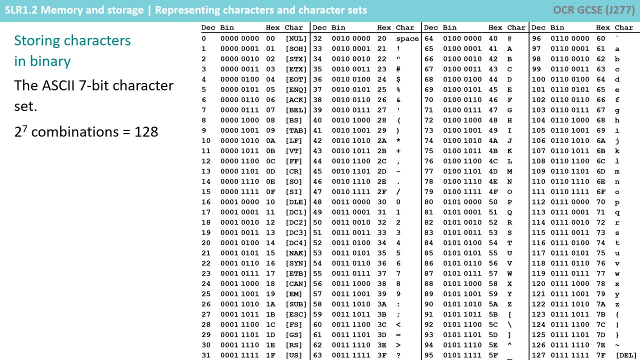 represent the capital letter A, then your computer must also recognize that same binary sequence as a capital letter A also. Therefore, character sets are agreed standards, an agreed way of numbering all the characters that computers use In the early days of computer science: ASCII or the American. 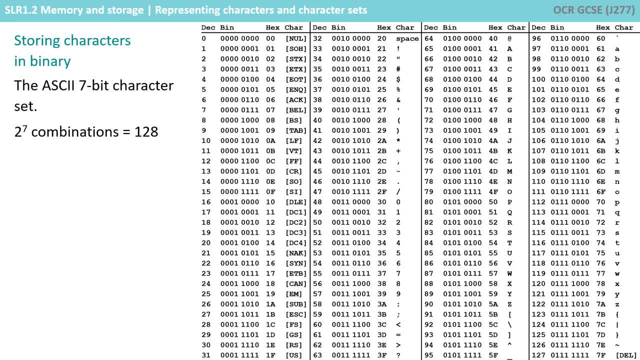 Standard Code for Information Interchange became an accepted standard. ASCII were a 7-bit character set. This means there were 2 to the power of 7 combinations of bits, which is 128 different combinations, and therefore it identified 128 characters and their binary codes or binary equivalents. 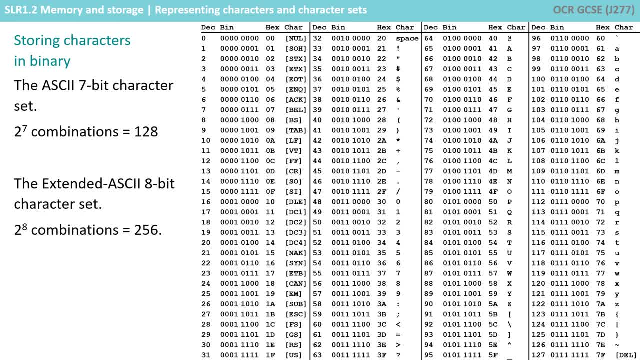 This was extended to an 8-bit code called extended ASCII, which provided for characters from some foreign languages. another useful graphical symbols: In 8 bits we have 2 to the power of 8 combinations and therefore 256 characters In ASCII. the numbers 0 to 31 were reserved for special. 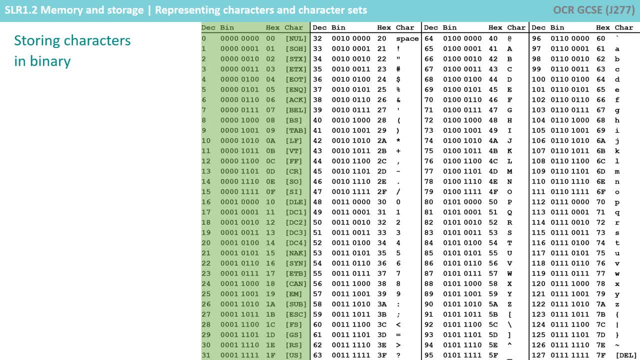 characters and instructions to the computer. So the recognizable part of the character set started of a space at number 32.. Purely out of interest, Character 7 caused your computer to beep. This was before the days of sound cards And character 13 was a new line character, which is why you often have to use commands like strip in programming when reading data from files to remove or strip these from the ends of lines of text. 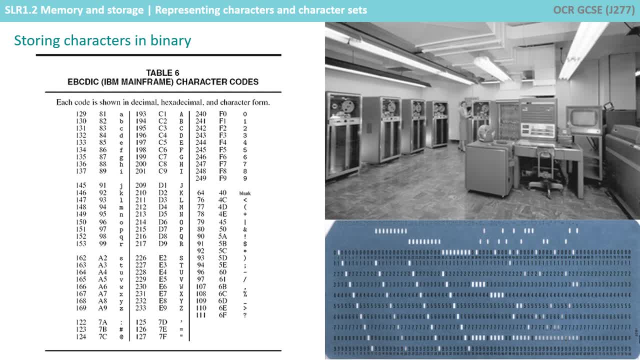 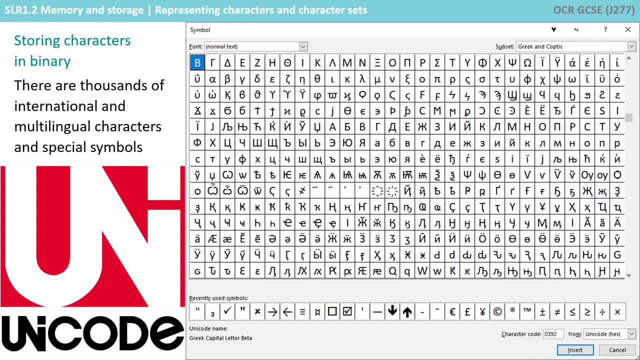 ASCII was not the only standard. Other character sets such as EBCDIC, also an 8-bit standard, were popular on mainframe computers and punch cards in the early days. Today, we have thousands of symbols we want to be able to store. 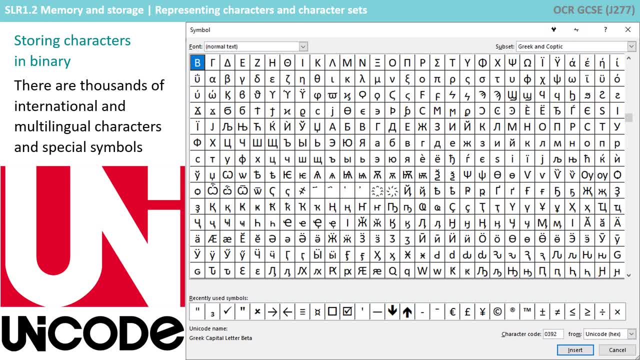 We want a fully international and multilingual character set which includes all the characters from every written language, historical scripts, plus more modern characters Such as emojis. These need to also conform to a standard, and this standard is known as Unicode or Universal Encoding.